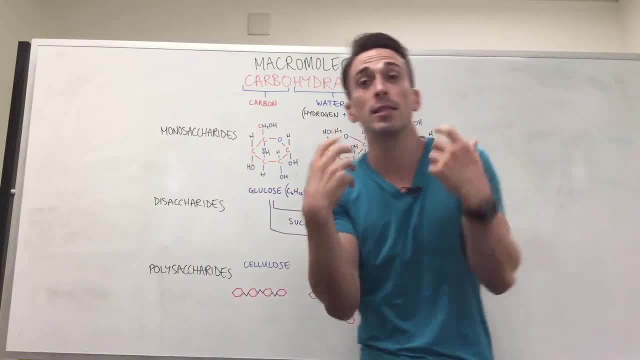 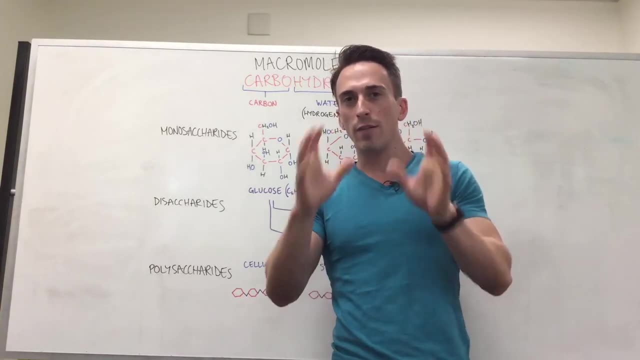 there's three main types of monosaccharides, what we term the simple sugars, and this includes glucose, fructose and galactose, which you've probably heard of before. Now, if you have a look, they are all made up of carbons, hydrogens and oxygens, and you'll actually find that they have 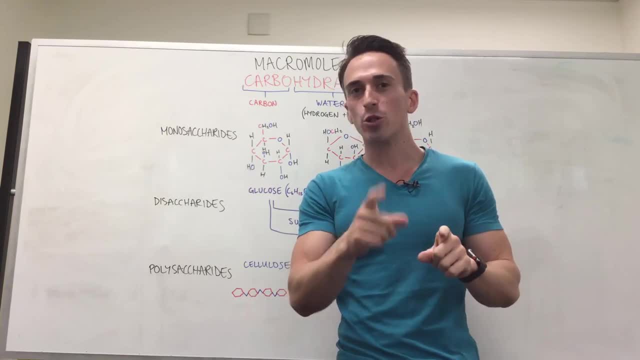 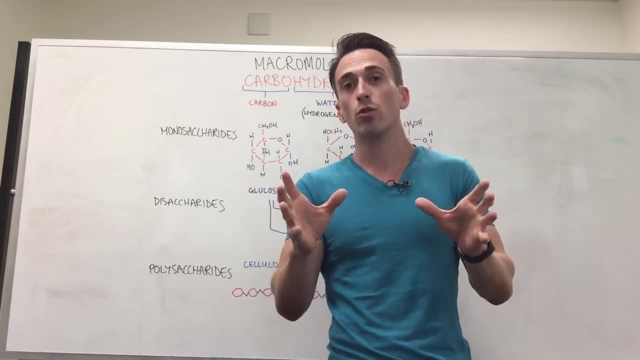 the exact same chemical formula, C6H12O6,, so there's six carbons, 12 hydrogens and six oxygens. The only difference between those three is that they're arranged differently. So glucose, which is our primary monosaccharide, 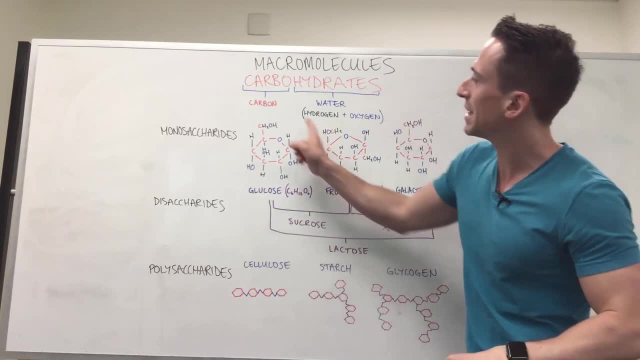 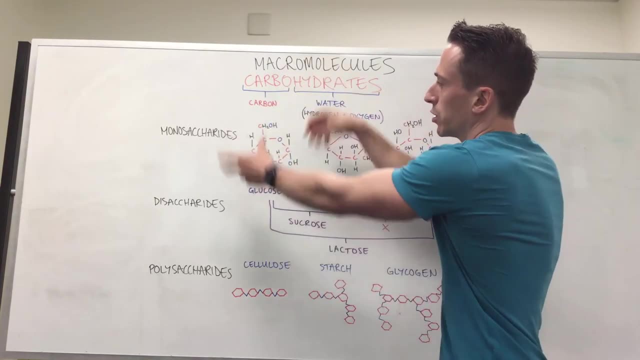 this is the main one we use to produce energy. you can see, this is the arrangement of all the carbons, all the hydrogens, all the oxygens. Okay, you can see the carbon ring with all the hydrogen and oxygens coming off. Then, when we look at fructose- still C6H12O6, it looks very similar. 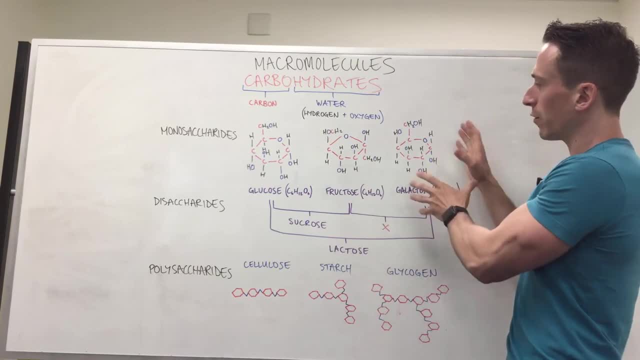 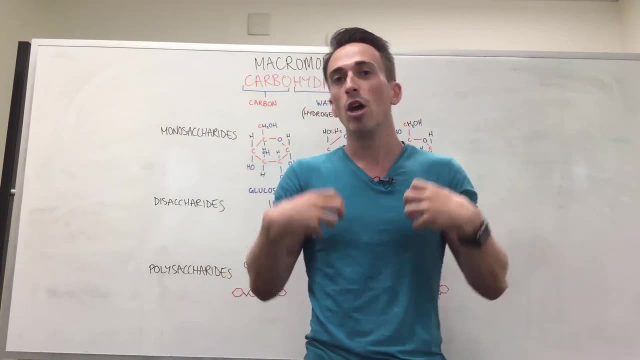 but there are a couple of differences. Same goes for galactose. very similar couple of differences. They're termed isomers of glucose. In actual fact, when you ingest foodstuffs, what will happen is once it's absorbed from the 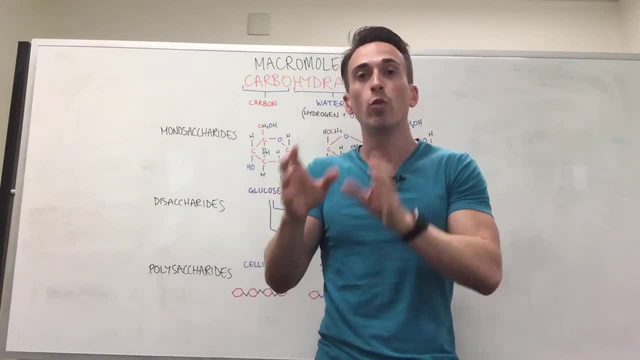 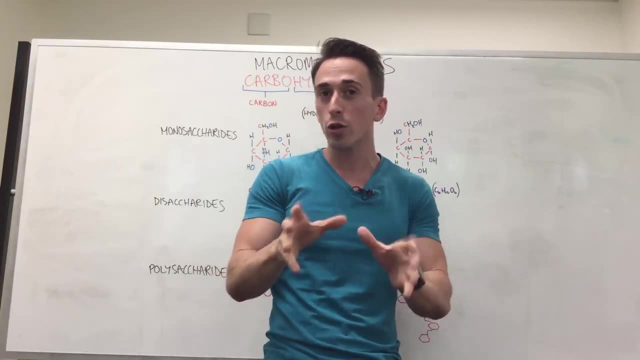 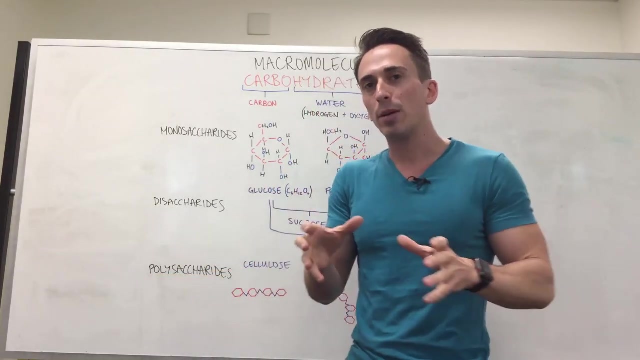 intestines into your bloodstream. it goes to your liver. your liver will convert galactose and fructose to glucose, either to use the glucose for energy or to store the glucose as a polysaccharide, which we term glycogen. but I'll get to that in one second. Now what can happen is you can ingest. 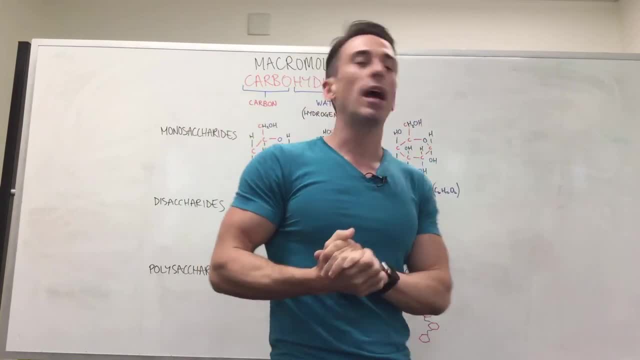 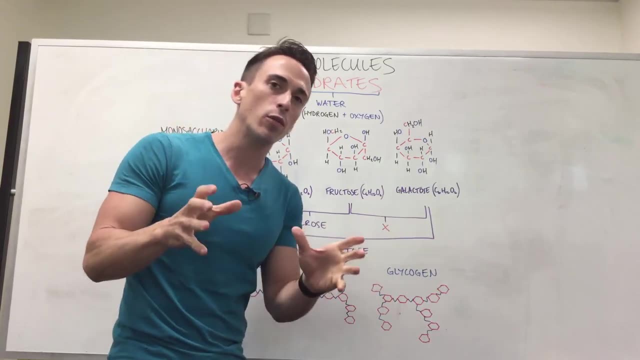 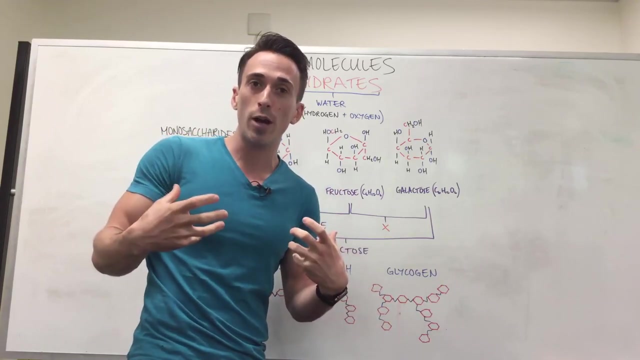 these carbohydrates, And when you have a look at these carbohydrates, for example, if you were to connect a glucose and a galactose together, you'd have to do it through a process called dehydration. You've heard that term before. dehydration, It means you don't have enough water in your body, right? So a dehydration. 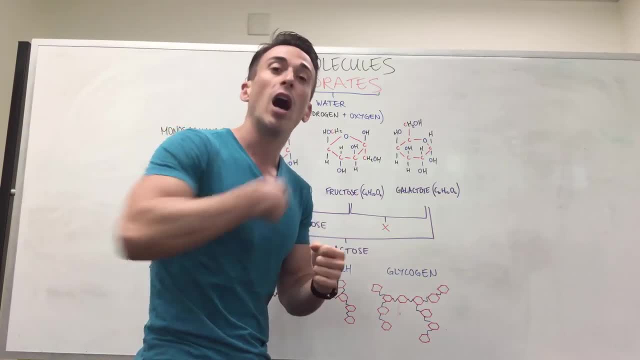 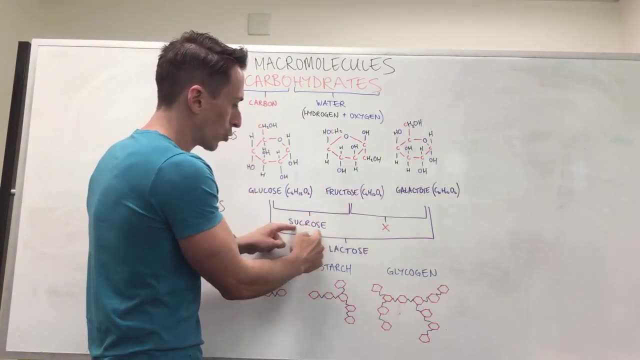 reaction simply means you release or you remove a water molecule from the reaction. It's very easy. If we first start off by connecting a glucose with a fructose, for example, that's termed sucrose. So that's what sucrose is. 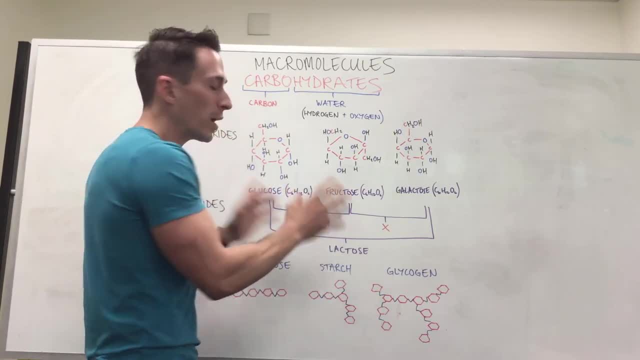 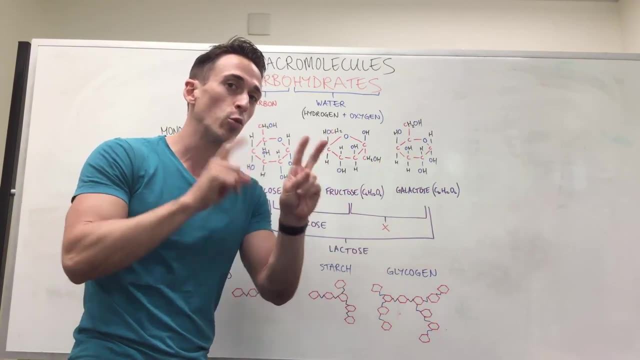 So that's what sucrose is: Simply a glucose connected to a fructose. The way you do it through a dehydration reaction is: water needs to be removed. Water is H2O- two hydrogen, one oxygen. There's a hydrogen, there's a hydrogen, there's an oxygen. So you remove them away and then those two. 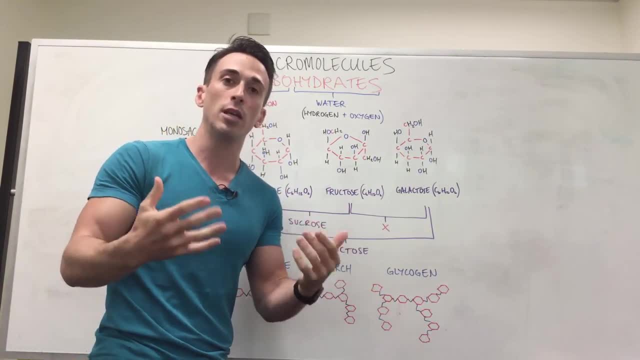 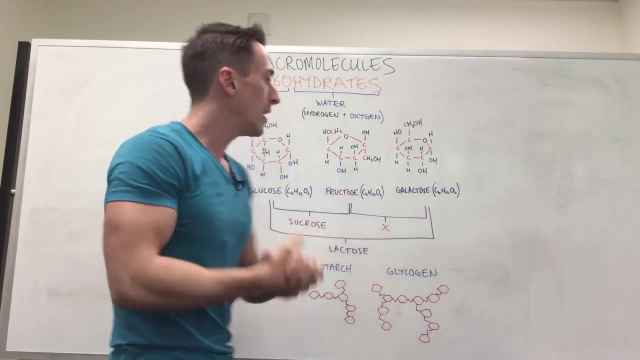 carbons can click together. That's how you form sucrose in a dehydration reaction. When you want to separate them, it's a rehydration reaction. You're going to put that water molecule back in. Now, if we were to connect glucose and galactose? 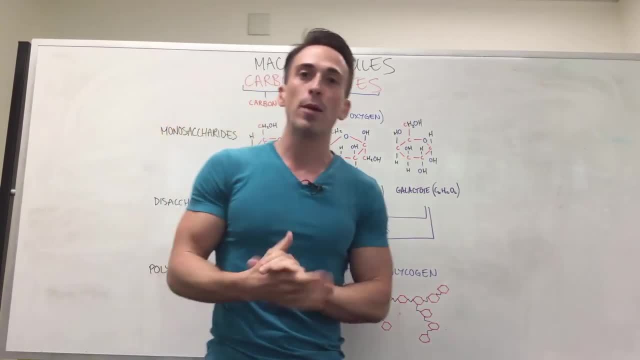 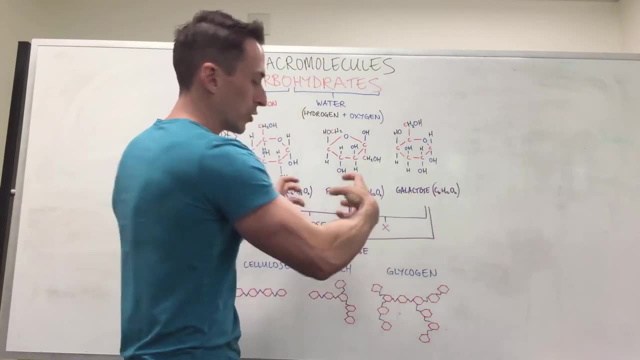 together we form something that's called lactose, And some people are lactose intolerant, which means when they ingest milk products, where you predominantly find glucose and galactose stuck together, you need an enzyme in your body that snips off that two bonds. 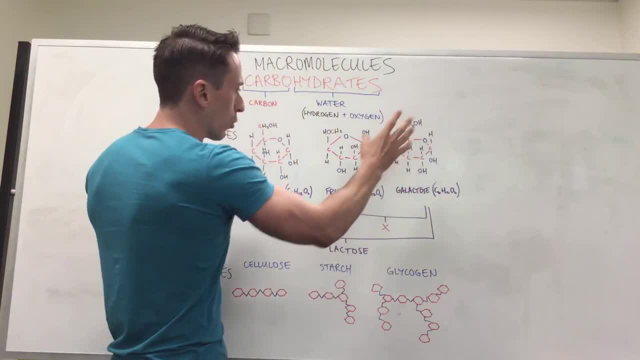 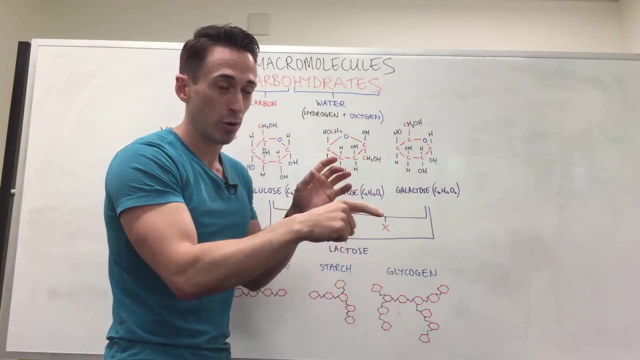 So remember, you got that water molecule, that's, you've taken away that water molecule. the carbons are held together. You need to rehydrate to break them apart and you need an enzyme to do this rehydration process When you're rehydrating that of lactose. 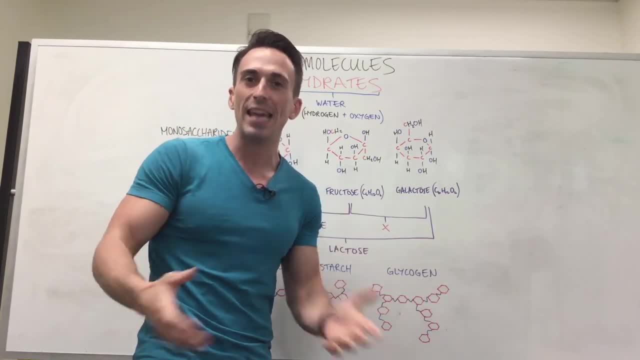 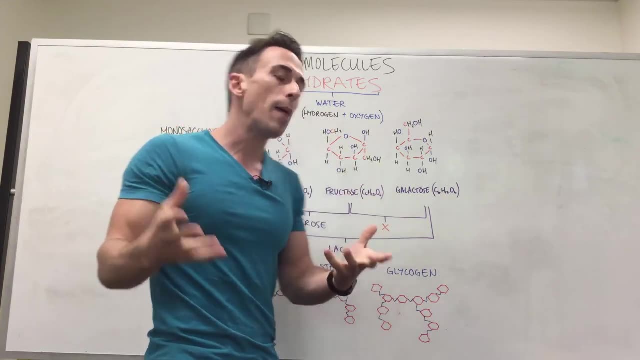 it's an enzyme called lactase A-S-E, And for some of us, we no longer produce lactase, and so we don't have the scissors that allows for us to cut that bond, And so what happens is the glucose and the galactose remain stuck together and continue to move through our intestines. We need to. 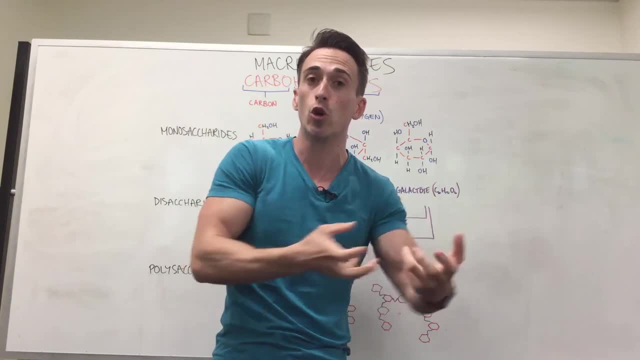 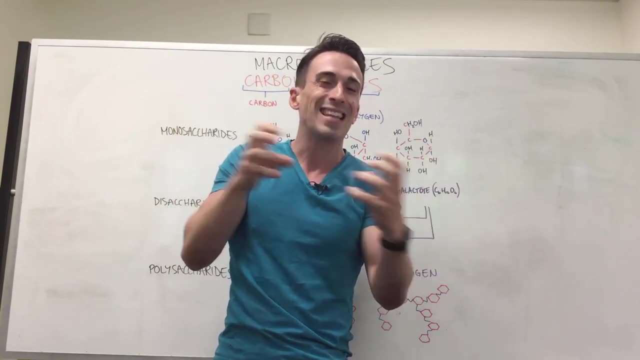 break this down into glucose and galactose in order for it to get absorbed from our intestines into the bloodstream so we can use it. If it doesn't snap apart through this hydration process, they stay together and it continues to move through the bloodstream, So we're going to 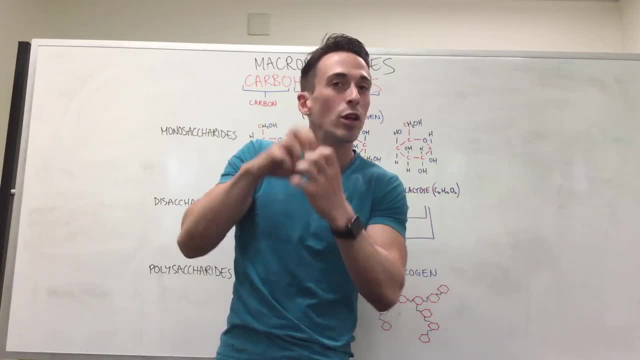 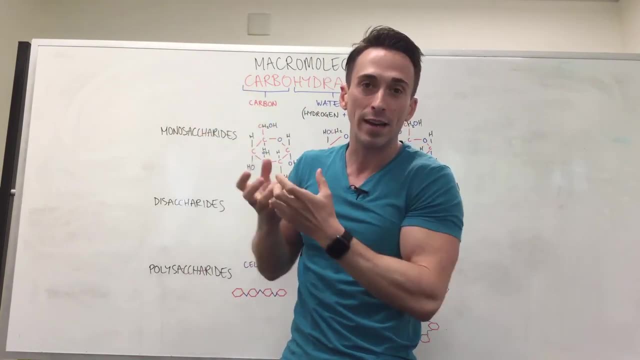 have to rehydrate through the digestive tract. Now this is a larger molecule, And when you've got large molecules moving in bulk through your intestines, it actually pulls water towards it. This is called an osmotic effect. And if it pulls water towards it now, your intestines are filled with. 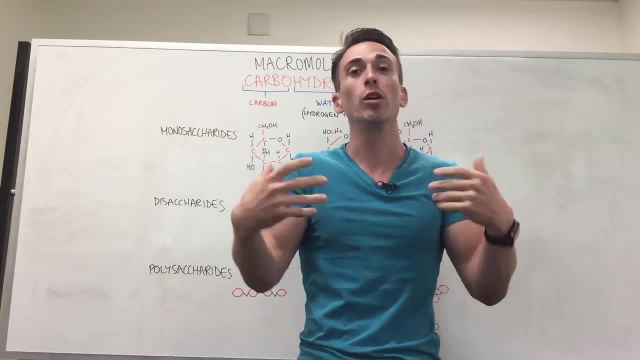 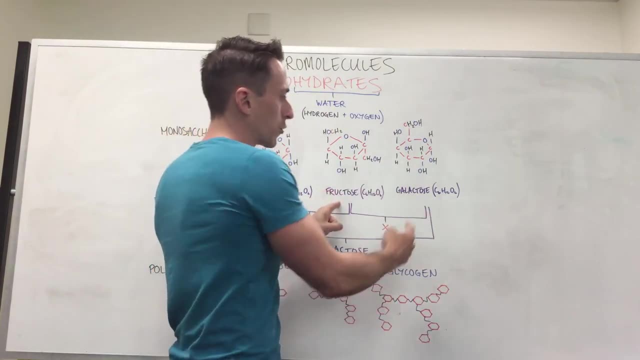 water and that goes out in the fecal material which we call diarrhea. So this is why lactose intolerance can result in diarrhea. Okay, The other thing is what if we were to click together fructose and galactose? Well, in actual fact, this doesn't happen, So you don't actually get a. 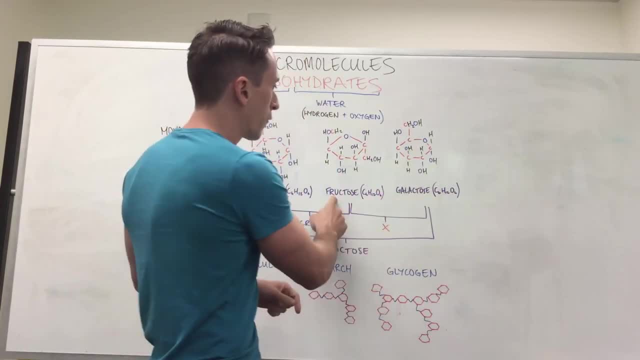 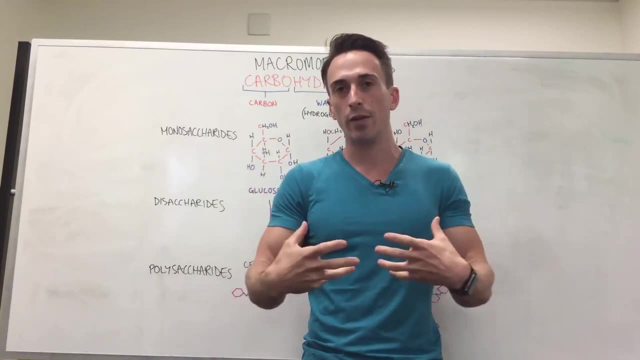 disaccharide, or fructose and galactose. now, like I said, fructose and galactose will ultimately turn in at the liver to glucose, and so now we've got a whole bunch of glucose molecules in our liver. we can either use it to form ATP energy or we can store it, and